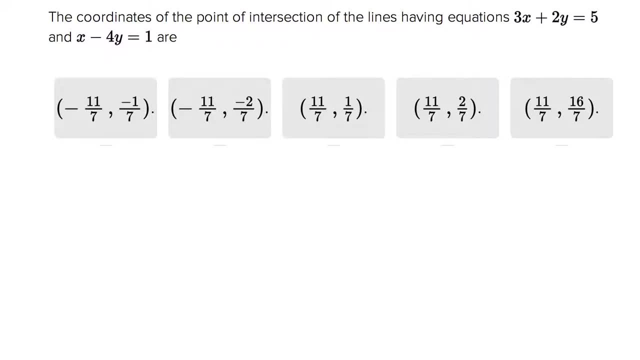 This is the real Tom Rose, and they're asking you what appears to be a geometry question. It uses the word coordinates, point of intersection lines. All that sounds very geometry, But at the end of the day, what they're basically giving you is two equations and two variables. 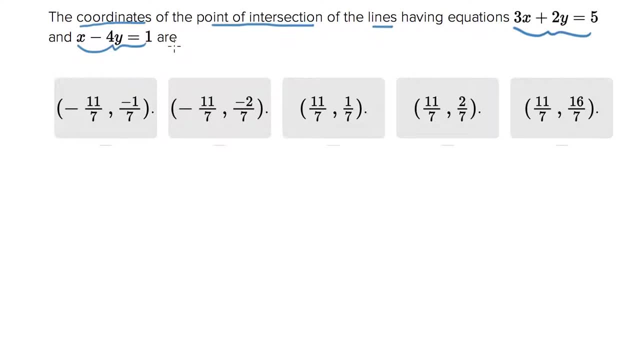 and they want the quote point of intersection. That's the same as saying the solution of these two equations. So another way to write this question would be: here's two equations with two variables. Solve it for x and y, right, And then take that solution and write it in order. 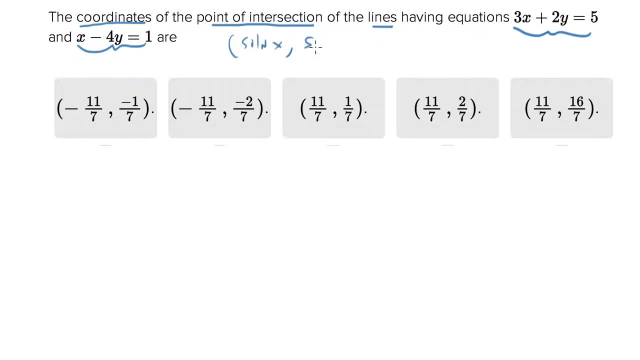 pair. So you have solution x, comma, solution y, and that's what we'll go hunt for in the answer choices. So this is really just an algebra question. So let's solve this the way we would solve any algebra question. Let's do a linear combination of these, So 3x plus 2y. 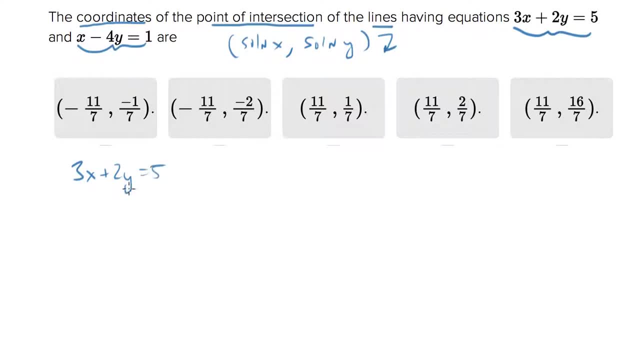 equals 5.. Unfortunately, we know it's going to work out terribly because you can just see the answer choices already. But plug onward. Let's take this equation- and I'm going to do some pre-work to make it line up more nicely- Let's multiply it all by 3.. Let's multiply every term. 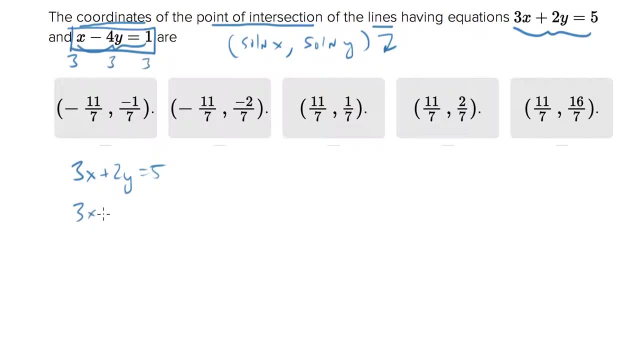 by 3.. So we'll end up with 3x minus 12y equals 3.. Subtract these equations from one another, So 3x minus 3x, those cancel. That's the whole beauty of this method. 2 minus negative 12y is 14y. 5 minus 3 is 2.. 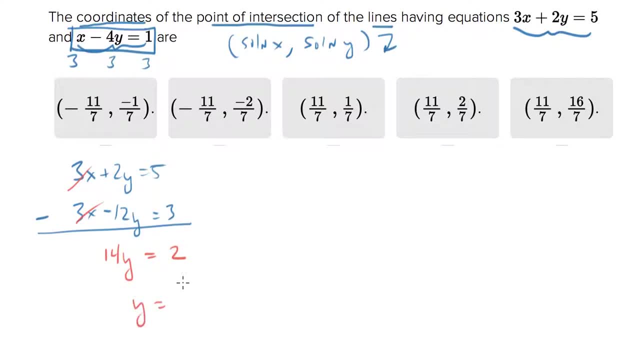 So y equals 2 over 14,, which is 1 over 7.. And oh, this worked out beautifully. Couldn't have planned it any better. We got the y-coordinate and if you go hunting in the answer choices, there's only one that works. 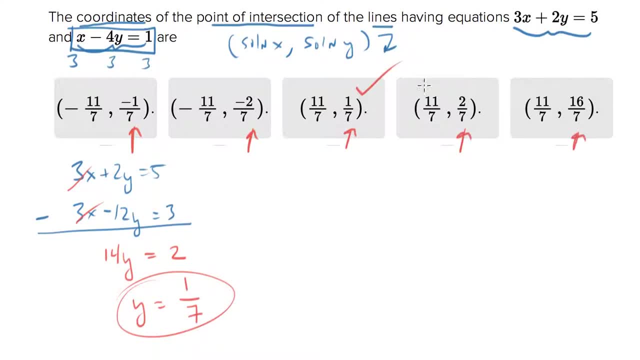 So we're done. It must be this one. If you want the x-coordinate, that's okay. You can still get it. You don't need it. But you could take that y, plug it into one of these equations, So you'd get.